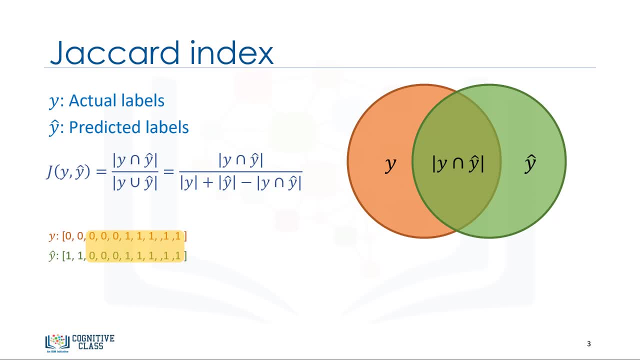 with eight correct predictions or eight intersections, the accuracy by the Jaccard index would be 0.66.. If the entire set of predicted labels for a sample strictly matches with the true set of labels, then the subset accuracy is 1.0.. Otherwise it is 0.0. Another way of looking at accuracy of 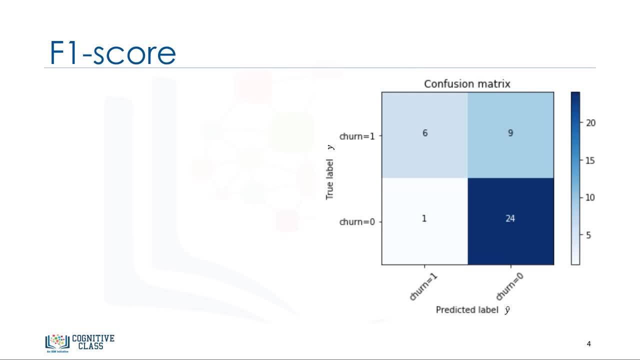 classifiers is to look at a confusion matrix, For example. let's assume that our test set has only 40 rows. This matrix shows the corrected and wrong predictions in comparison with the actual labels. Each confusion matrix row shows the actual true labels in the test set. If the test set has only 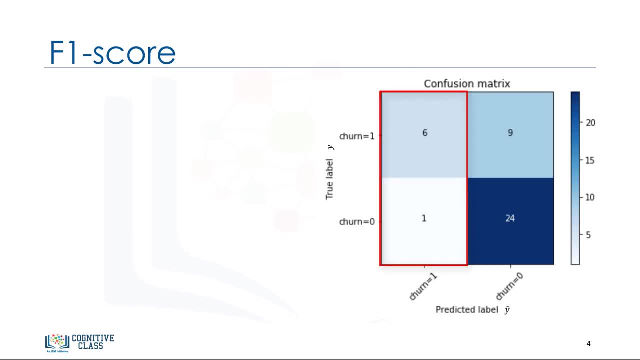 one column. then the columns show the predicted labels by classifier. Let's look at the first row. The first row is for customers whose actual churn value in the test set is 1.. As you can calculate, out of 40 customers, the churn value of 15 of them is 1. And out of these 15,. 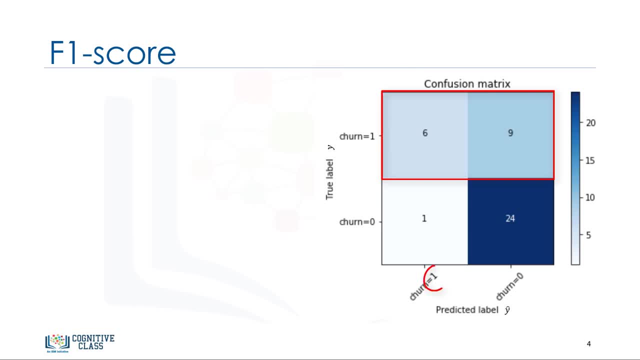 the classifier correctly predicted 6 of them as 1 and 9 of them as 0. This means that for 6 customers the actual churn value was 1 in the test set and the classifier also correctly predicted those as 1.. 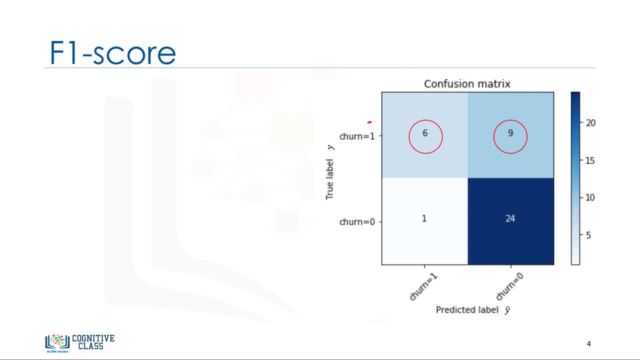 However, while the actual label of 9 customers was 1,, the classifier predicted those as 0,, which is not very good. We can consider this as an error of the model for the first row. What about the customers with a churn value 0?? Let's look at the second row. It looks like there. 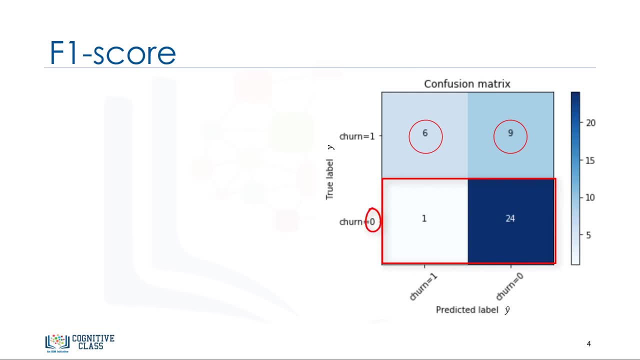 were 25 customers whose actual churn value was 1, so we need a different classification for 0.. For the churn data customers whose churn value is 0. The classifier correctly predicted 24 of them as 0 and one of them wrongly predicted as 1.. So it has done a good job in predicting the customers with a churn value. 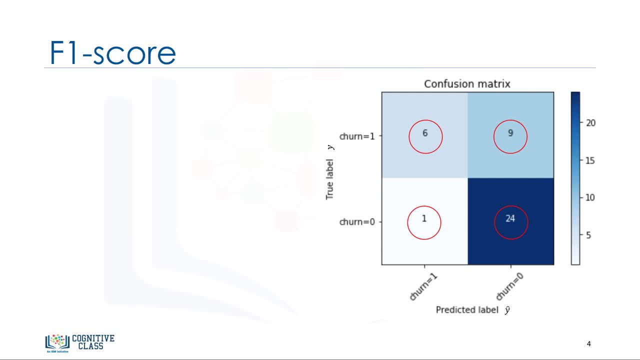 of 0.. A good thing about the confusion matrix is that it shows the model's ability to correctly predict or separate the classes. In the specific case of a binary classifier such as this example, we can interpret these numbers as the count of true positives, false positives, true negatives. 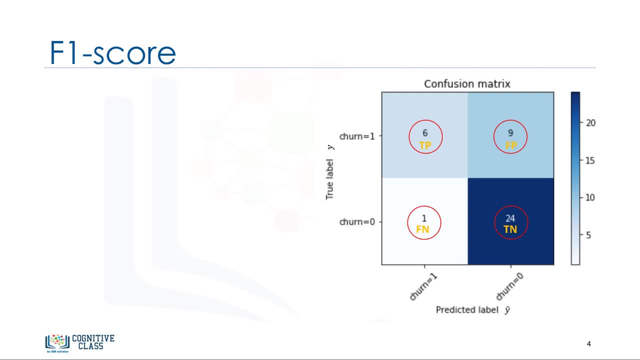 and false negatives. Based on the count of each section, we can calculate the precision and recall of each label. Precision is a measure of the accuracy provided that a class label has been predicted. It is defined by precision. equals true positive divided by true positive plus false. 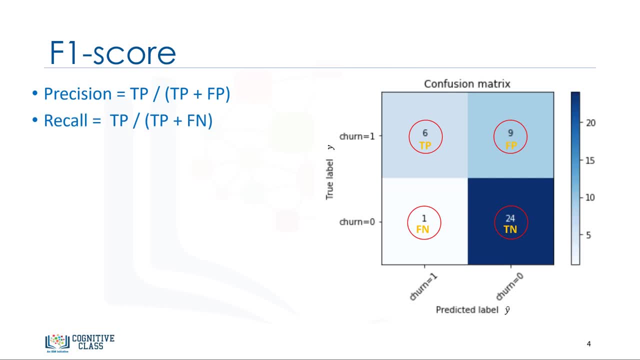 positive And recall is the true positive rate. It is defined as: recall equals true positive divided by true positive plus false negative. So we can calculate the precision and recall of each class. Now we're in the position to calculate the F1 scores for each label. 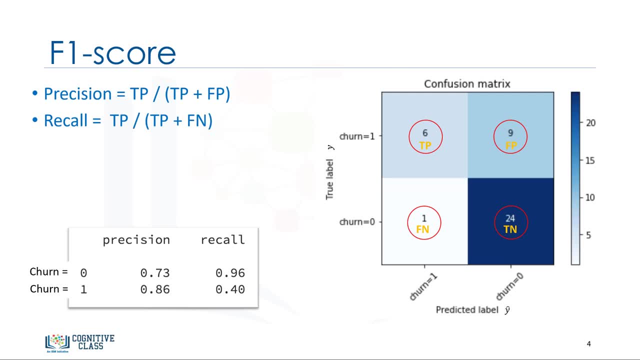 based on the precision and recall of that label. The F1 score is the harmonic average of the precision and recall, where an F1 score reaches its best value at 1,, which represents perfect precision and recall, and its worst at 0.. It is a good way to show. 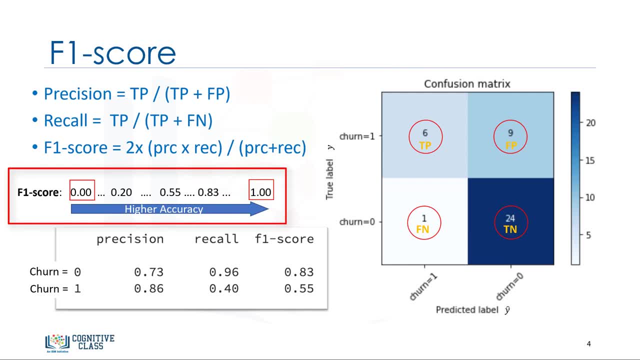 that a classifier has a good value for both recall and precision. It is defined using the F1 score equation. For example, the F1 score for class 0, ie churn equals 0, is 0.83, And the F1 score for class 1, ie churn, equals 1, is 0.55. 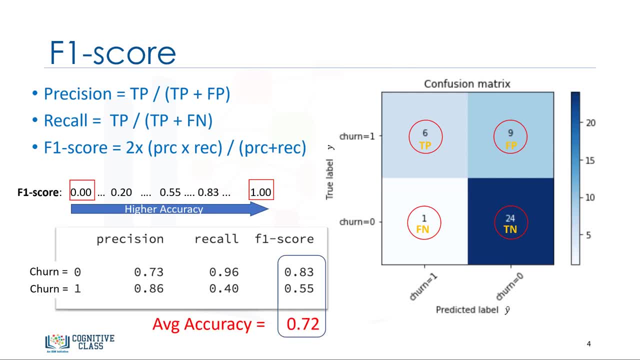 And finally, we can tell: the average accuracy for this classifier is the average of the F1 score for both labels, which is 0.72 in our case. Please notice that both Jackard and F1 score can be used for multi-class classifiers as well, which is out of scope for this course. 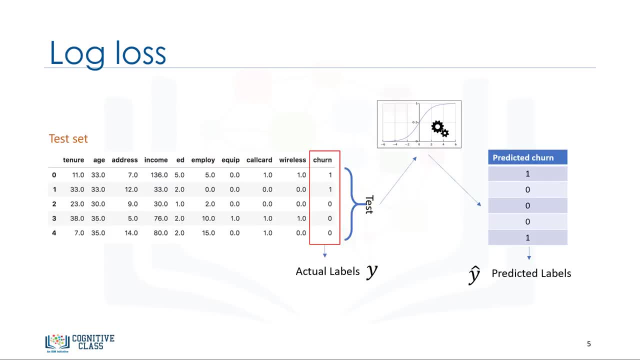 Now let's look at another accuracy metric for classifiers. Sometimes the output of a classifier is the probability of a class label instead of the label. For example, in logistic regression the output can be the probability of customer churn, ie yes, or equals to 1.. 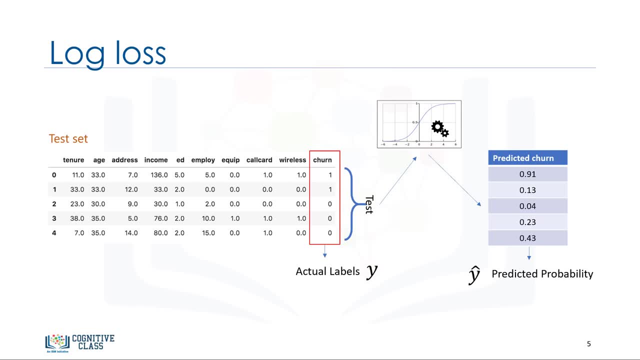 This probability is a value between 0 and 1.. Logarithmic loss, also known as log loss, measures the performance of a classifier where the predicted output is a probability value between 0 and 1.. So, for example, predicting a probability of 0.13 when the actual label is 1 would be bad and would result in a high log loss.